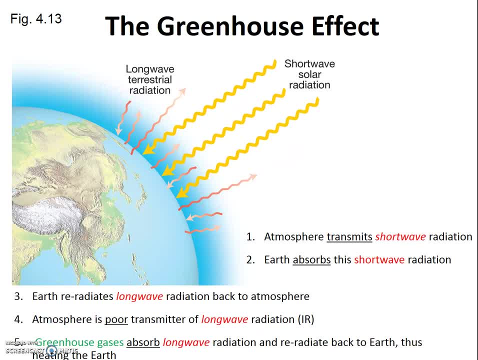 not able to escape the troposphere, and the troposphere heats up. You should be able to talk your way through this process and also identify major greenhouse gases. You should be able to myself, but also include important person and crudely important speaker. 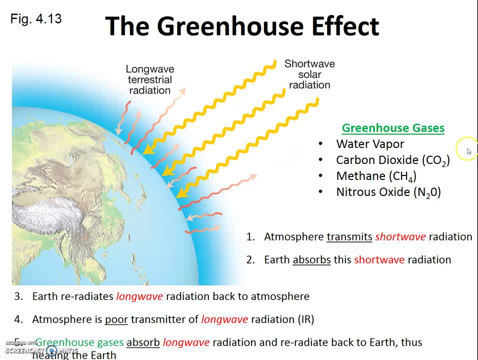 겠어 and give sources for each jakus. he ended us a prospect of those sources you generated, sources especially for these three here: carbon dioxide, methane and nitrous oxide, probably the three most important greenhouse gases that humans have dramatically increased in the troposphere. 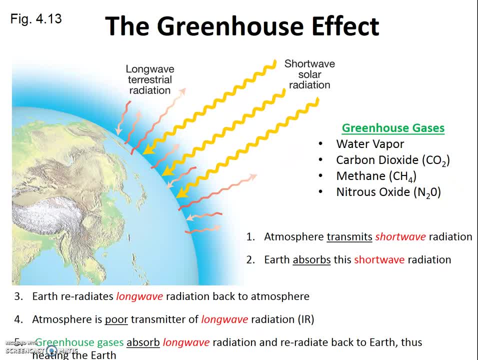 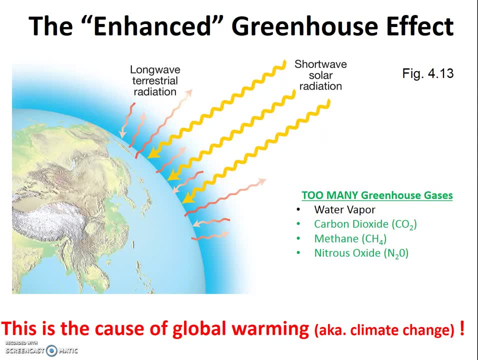 to practice and for which, as we just noted, the greenhouse effect is a natural process. However, the problem is that humans are adding extra greenhouse gases into the atmosphere, which result in more heat retention and rising tropospheric temperatures. Sometimes, this process is referred to as the enhanced 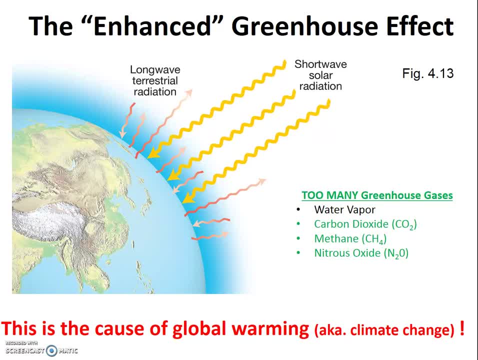 greenhouse effect, because it is essentially extra warming caused by the addition of anthropogenic, human-generated greenhouse gases. The addition of these extra anthropogenic greenhouse gases is the cause of global warming. Notably, the more appropriate term for global warming is climate. 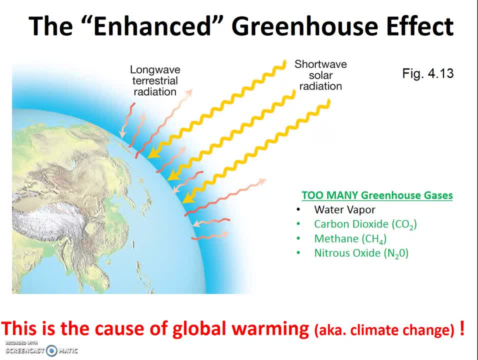 change, as this general term is able to encompass the many diverse effects we expect to see result from the warmer tropospheric temperatures. For example, some regions, Europe notably, will actually get cooler. We will discuss climate change in more detail when we cover climate in a few weeks. 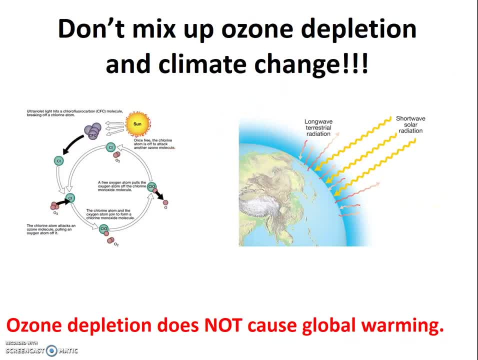 Lastly, and very importantly, don't mix up ozone depletion- that we covered in Chapter 3, and climate change, which we're introducing now. They are very different phenomena and they're not related in the way that many people think. Also, ozone depletion is a stratospheric phenomena, whereas climate change. 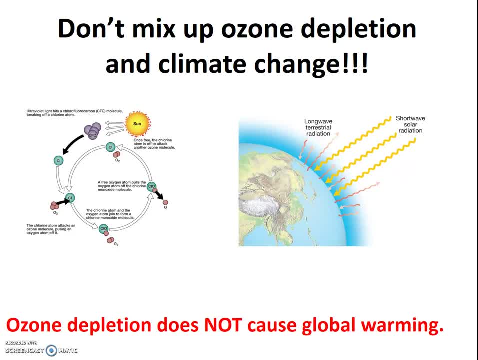 is a tropospheric phenomena. Importantly, ozone depletion does not mix up ozone depletion and ozone depletion does not cause global warming or climate change. This is important. You should say this aloud to yourself: Ozone depletion does not cause climate change. Many students